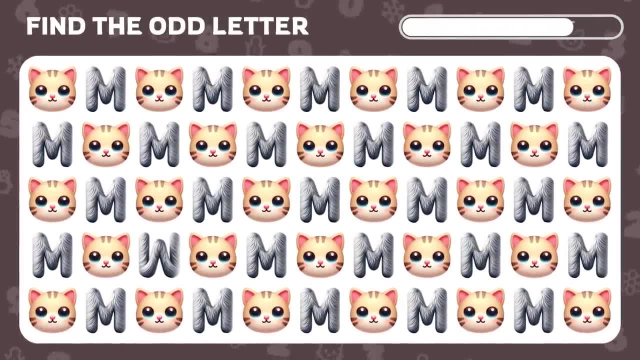 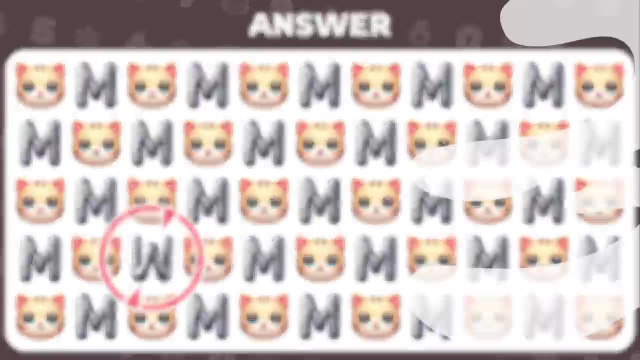 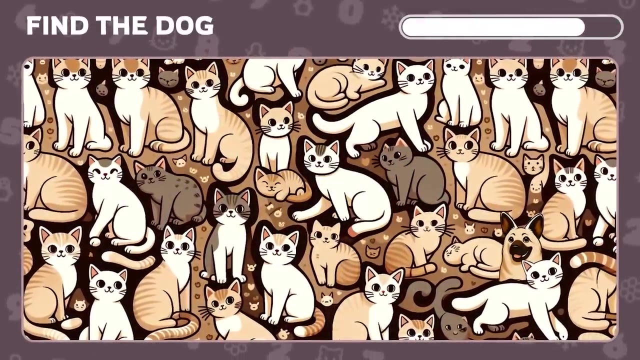 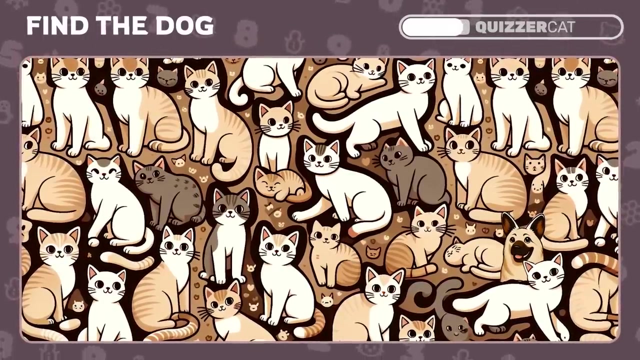 Can you find the different letter among these cat emojis? Correct, It's the letter W, Level 4.. Try to find the dog among all these cats. Try to find the dog among all these cats Right here. Great, the dog is hiding on the right. 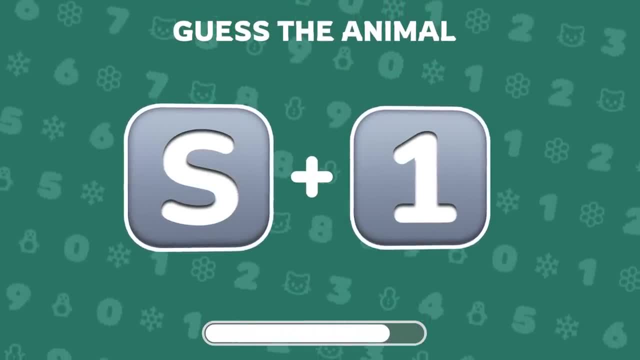 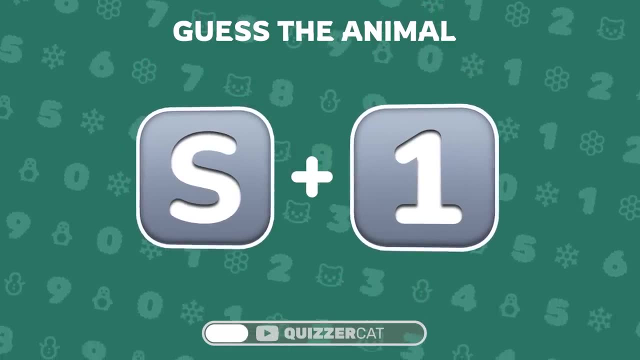 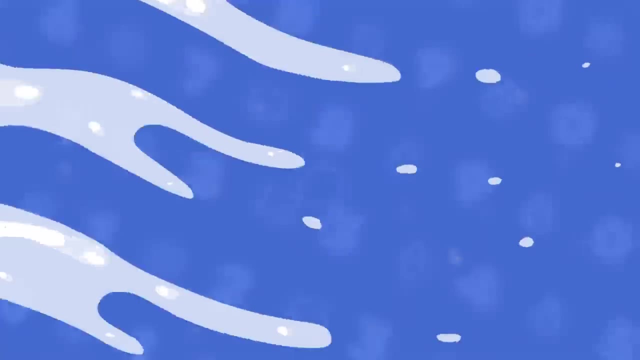 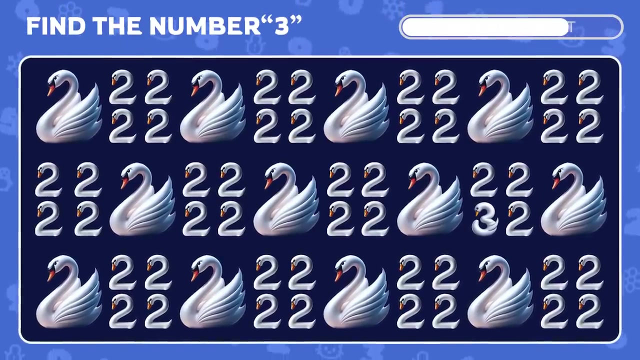 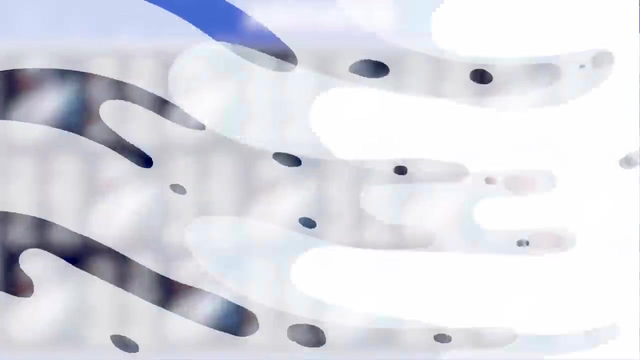 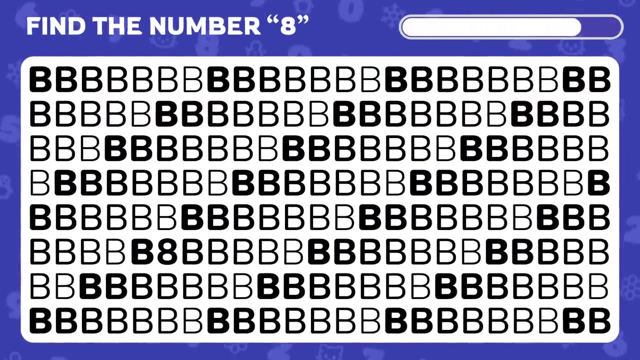 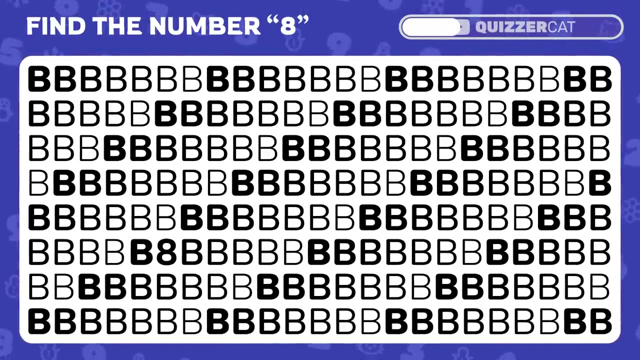 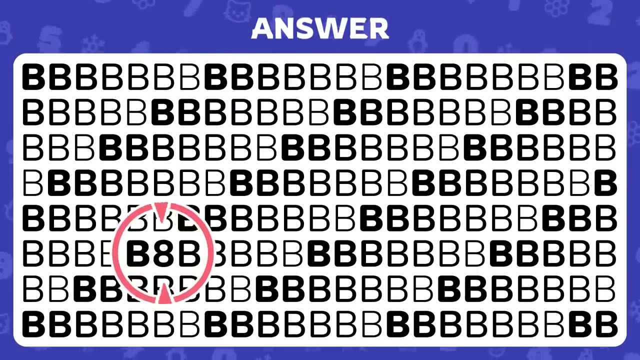 Guess the animal only by these two symbols. Guess the animal only by these two symbols. Right here It's swan. Easy, easy, right now, among these swans, try to find the number three. and there, it is nice job: find the number eight among lots of letter B. yes, the number eight is right here, let's. 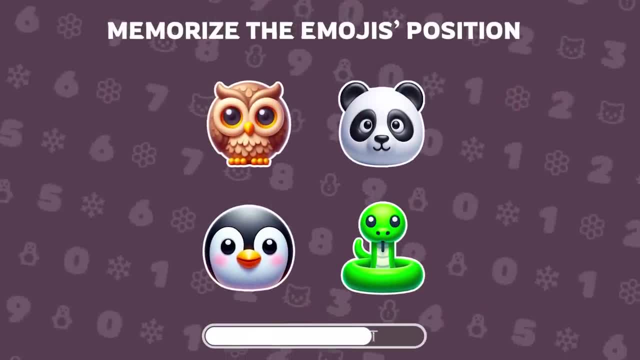 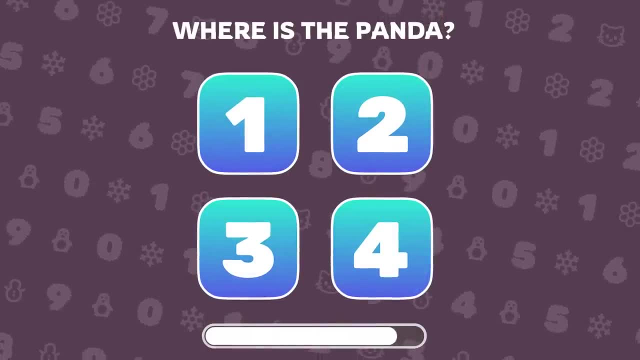 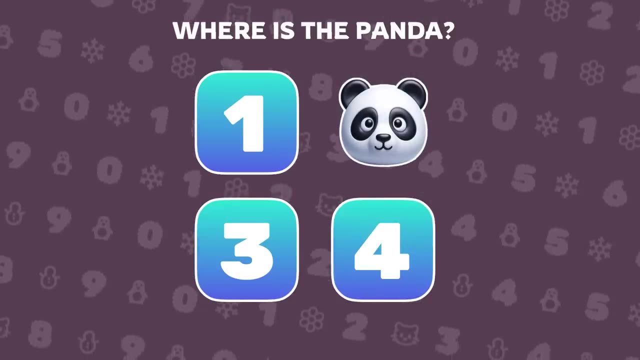 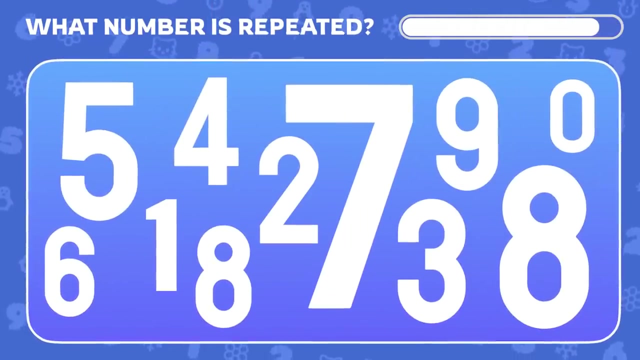 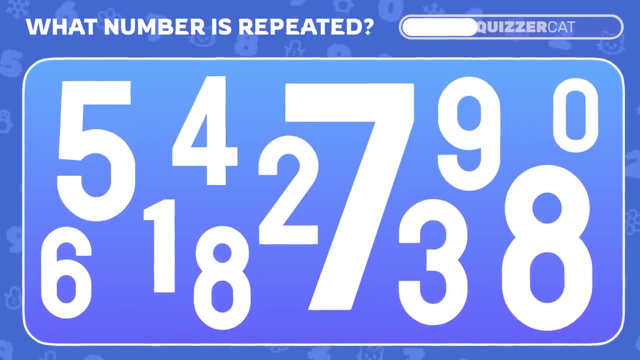 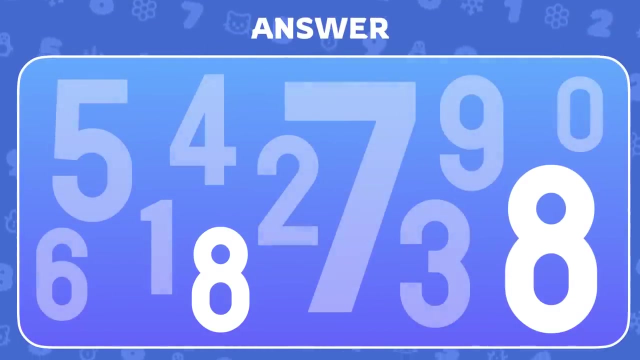 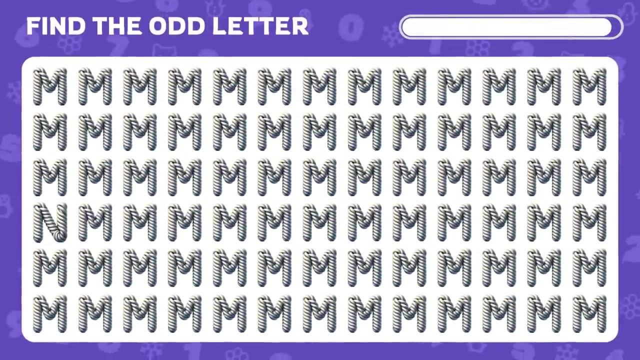 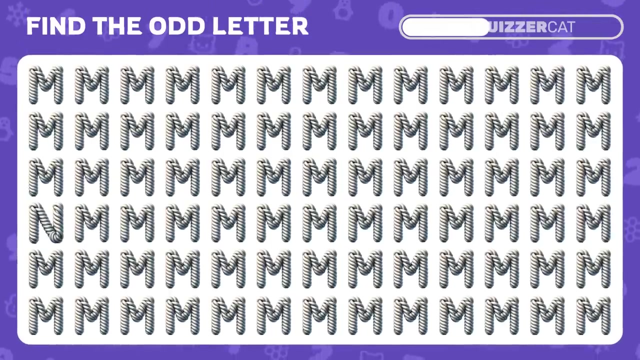 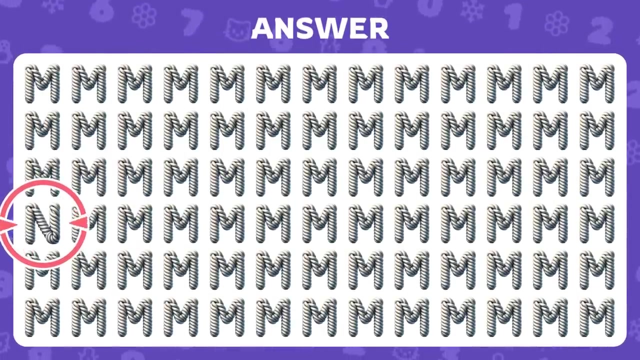 test your photographic memory. remember the position of all four emojis and now guess where's the panda hiding. yes, panda is under number two. next challenge: find the number that appears twice. excellent, it's the number eight. one more easy level: try to find the different letter. yes, it's the letter N. 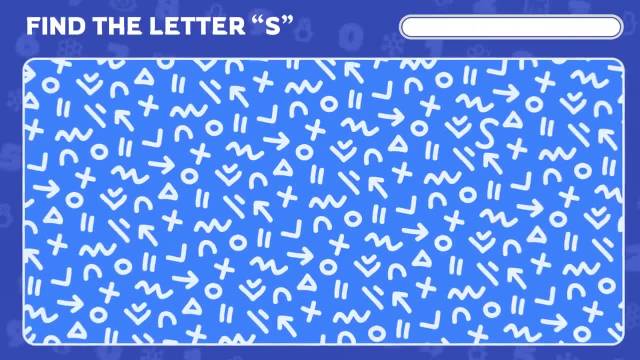 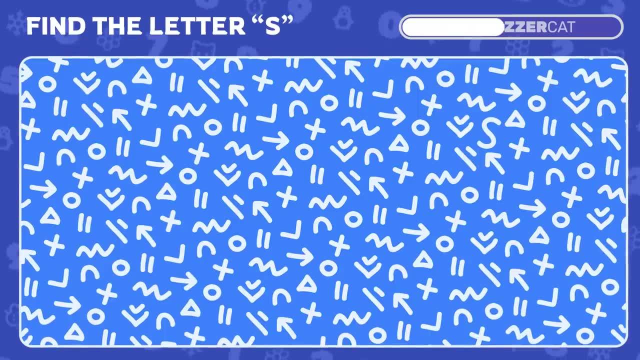 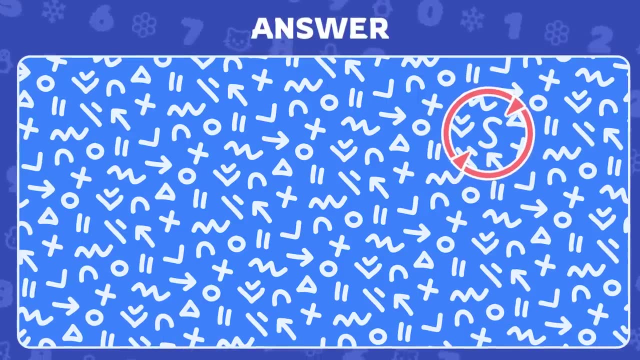 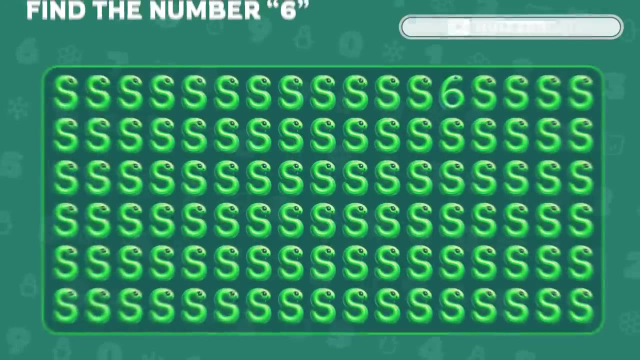 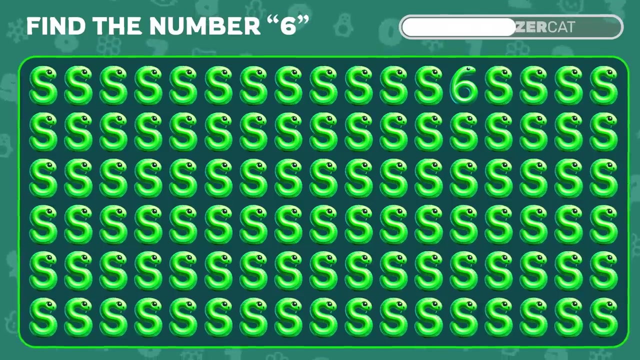 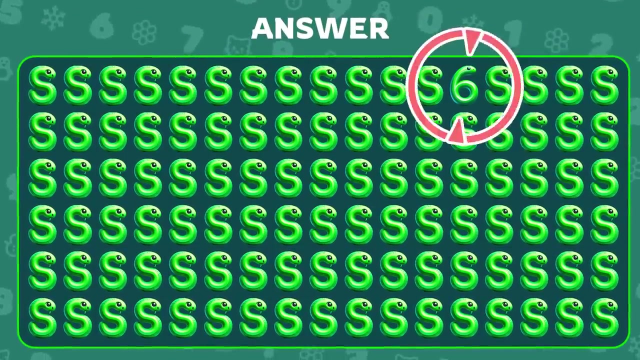 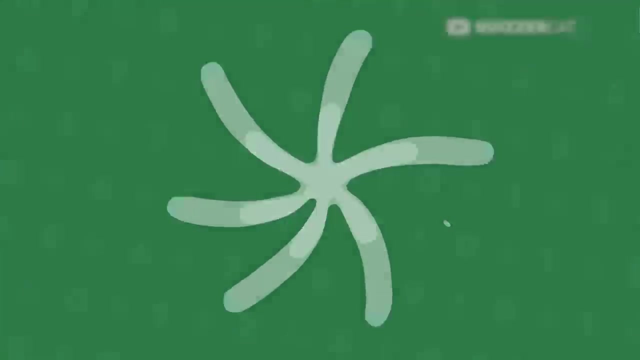 stepping up to medium difficulty. can you find the letter S in this image? there, it is not too hard. now try to find the number six among the letter S's step up to medium difficulty. can you find the letter S in this image? Number 6 is in the first row. 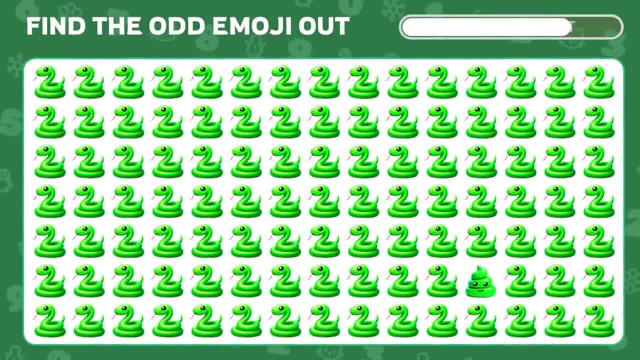 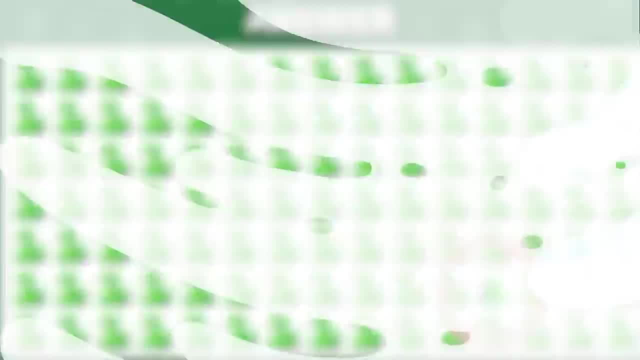 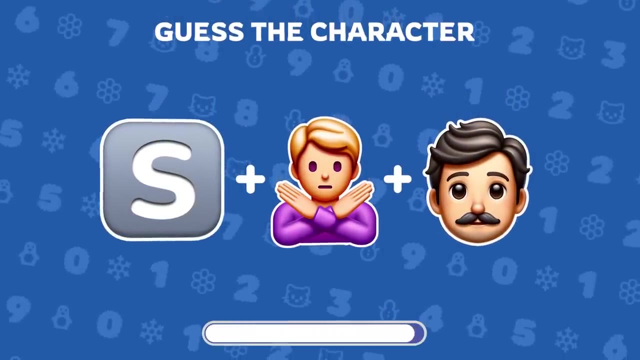 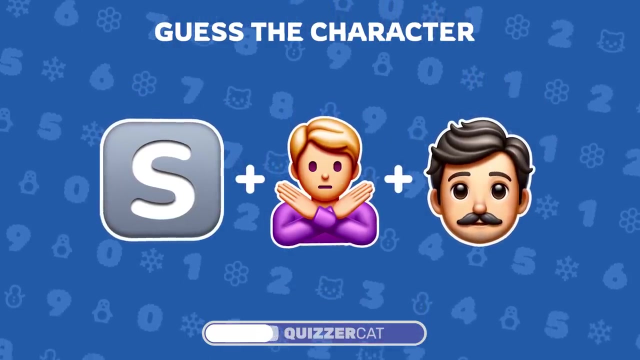 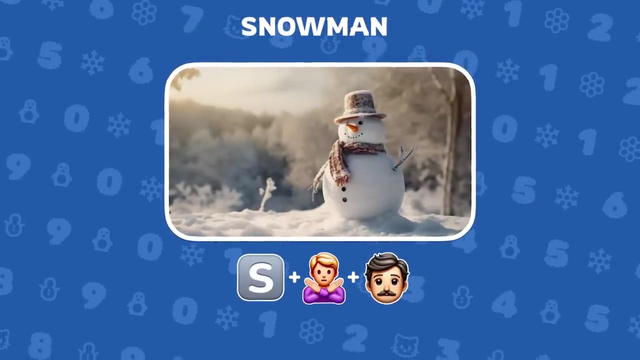 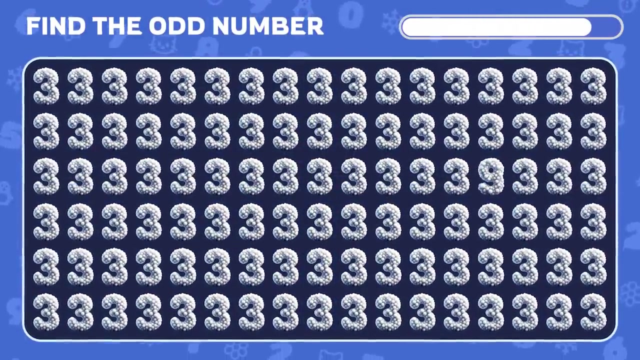 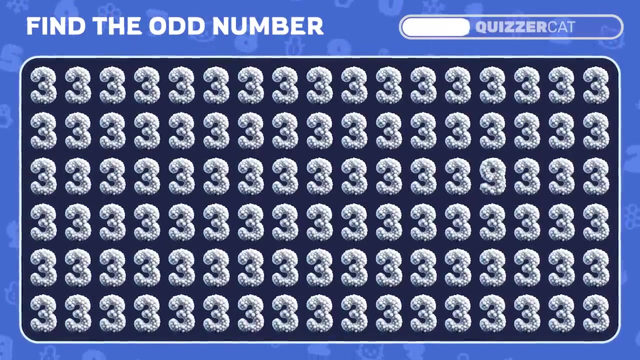 Another level with snakes. Find the different emoji. Aha, It's the poop emoji. Guess the character from these three emojis? Oh, Correct answer is snowman. Now find the snow-covered number that differs from the rest. It's the number 9.. 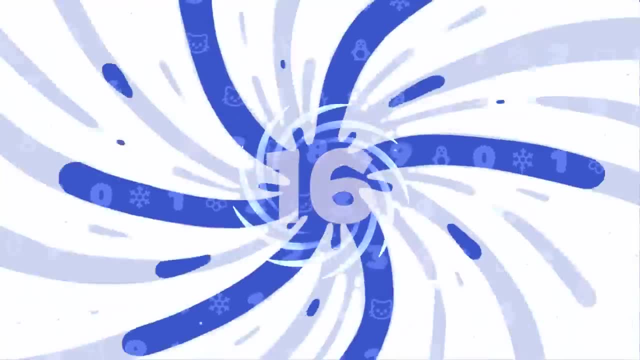 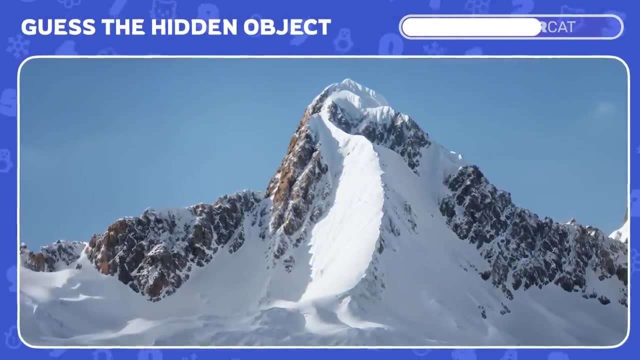 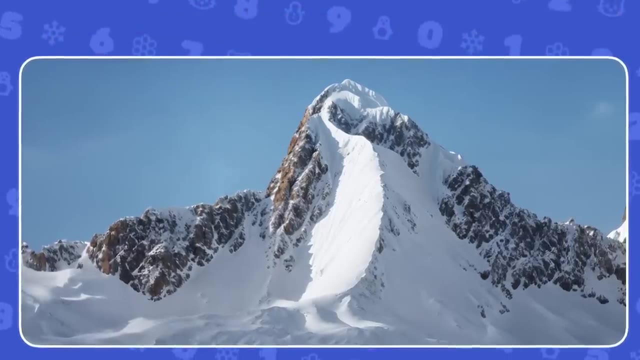 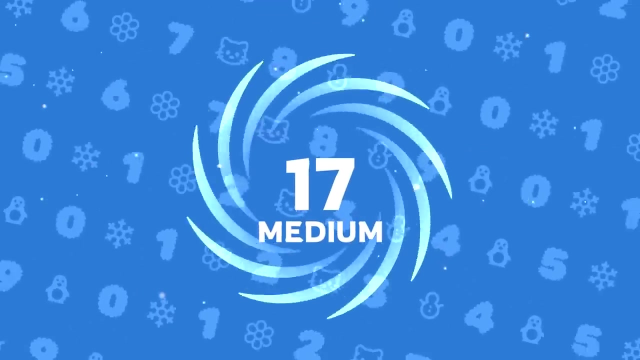 Optical illusion level. Who's hiding among these snowy mountains? Right, It's a penguin. Try to find the different emoji among the snowflakes in the first row. Now find the different emoji. Try to find the different emoji among the snowflakes in the first row. 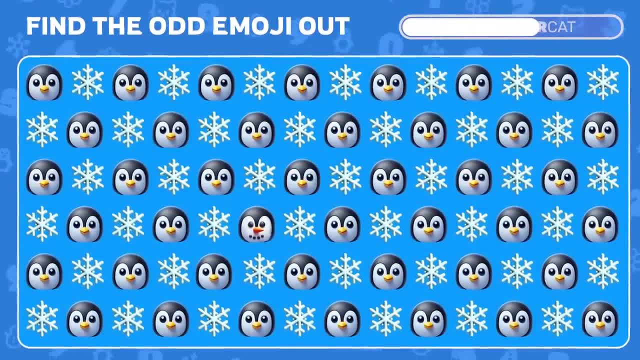 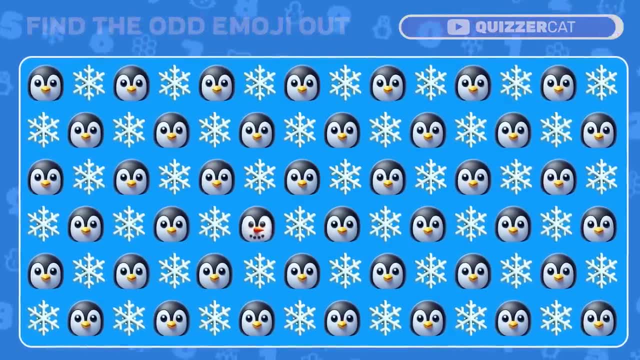 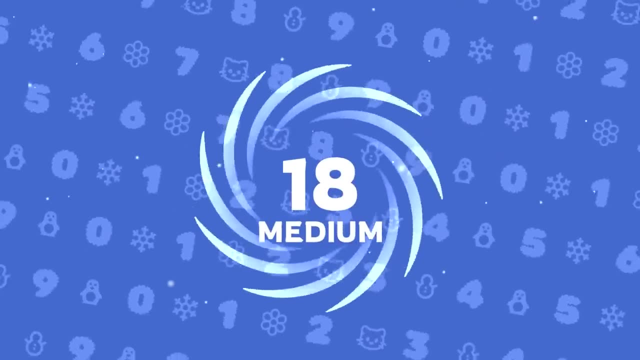 Now find the different emoji among the snowflakes in the first row. Try to find the different emoji among the snowflakes and penguins. Try to find the different emoji among them. Wow, It's a snowman. Get to know, Snowman. 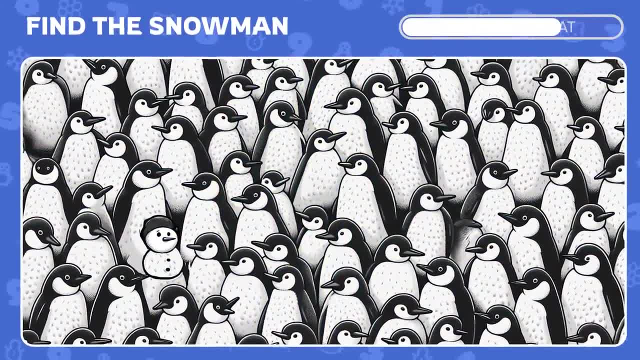 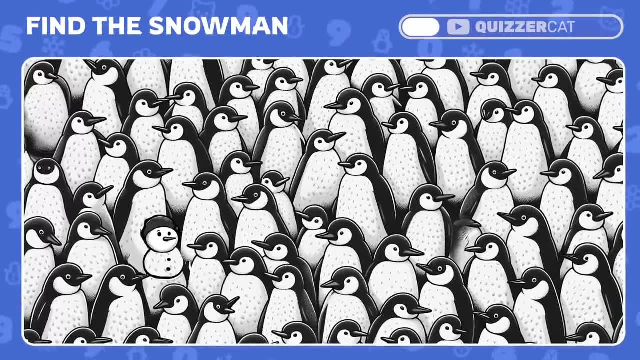 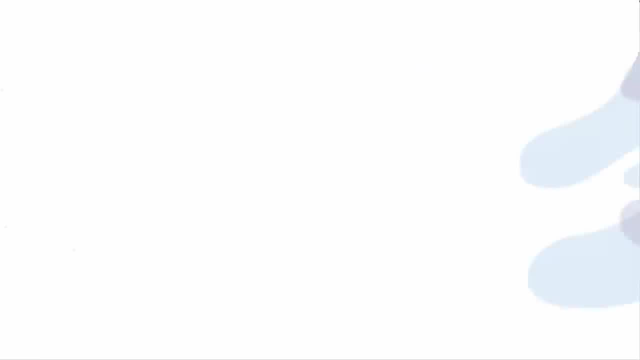 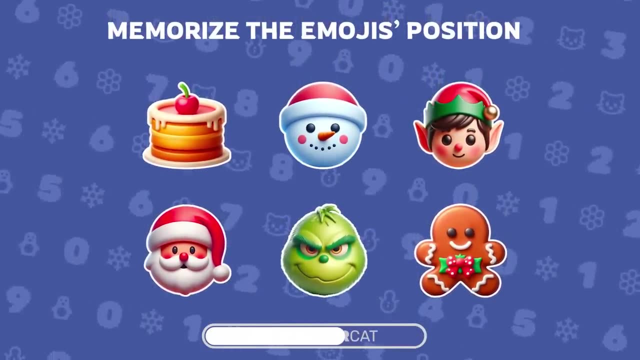 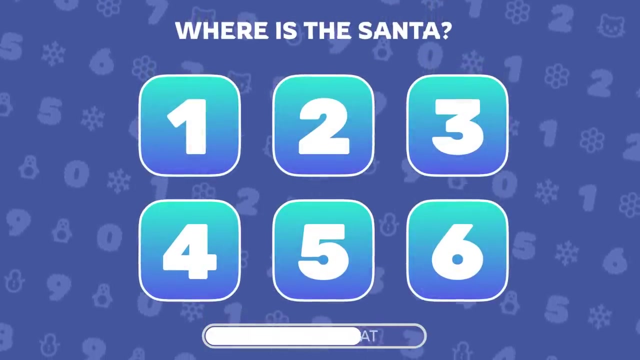 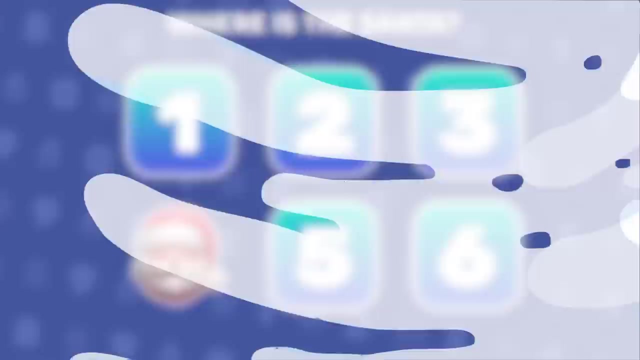 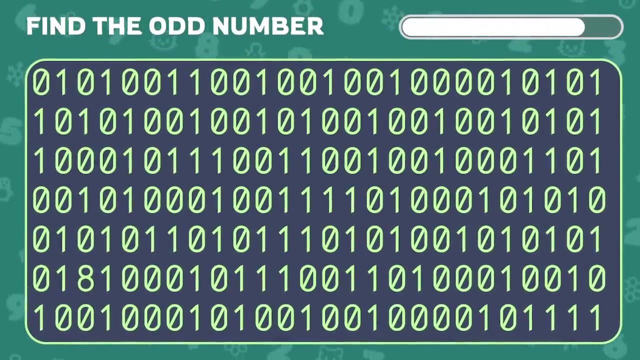 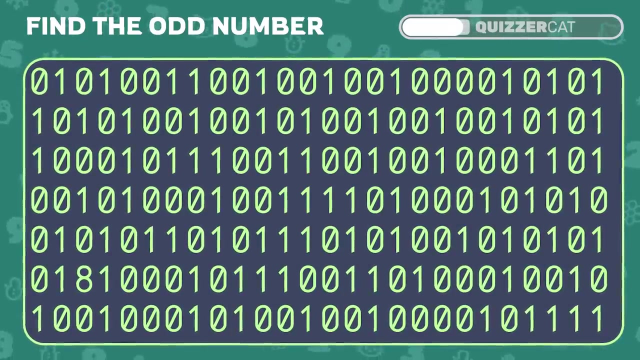 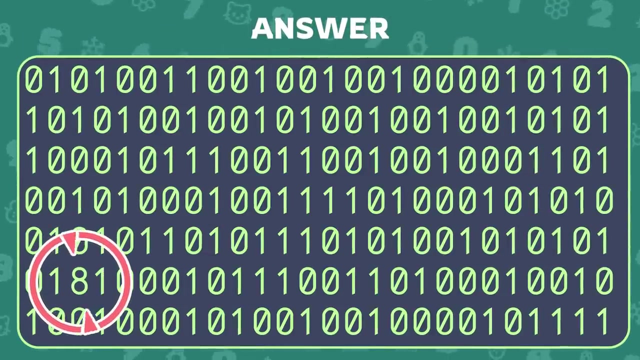 Now find the snow man among lots of penguins Found 21.. and there it is. remember the positions of these six emojis. which number is Santa hiding under? what Santa is under? number four: find the different number in this binary code. it's the number eight. 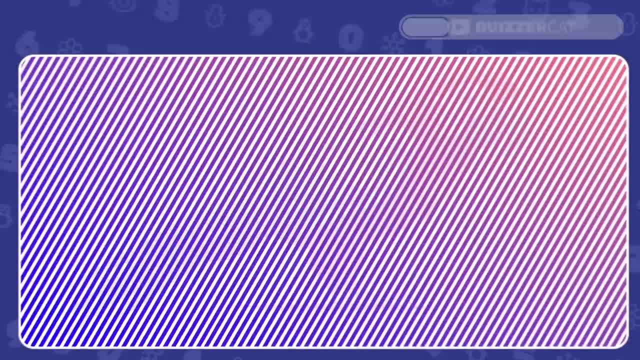 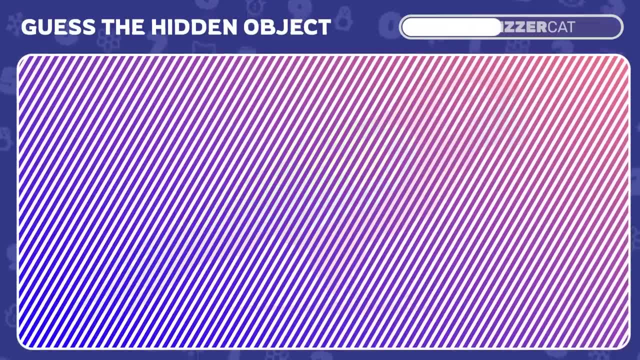 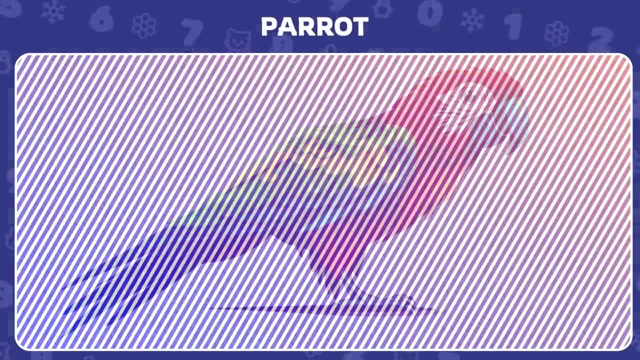 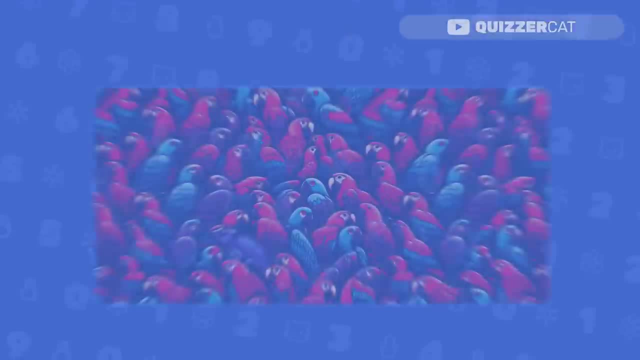 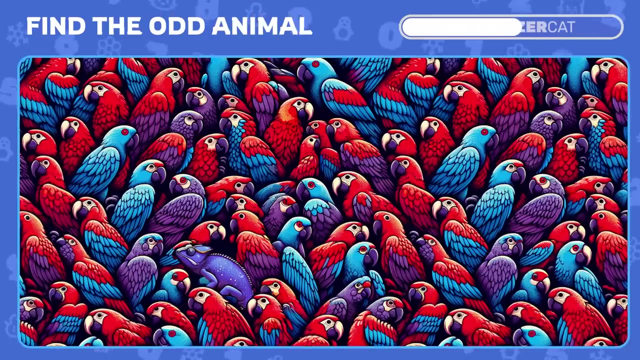 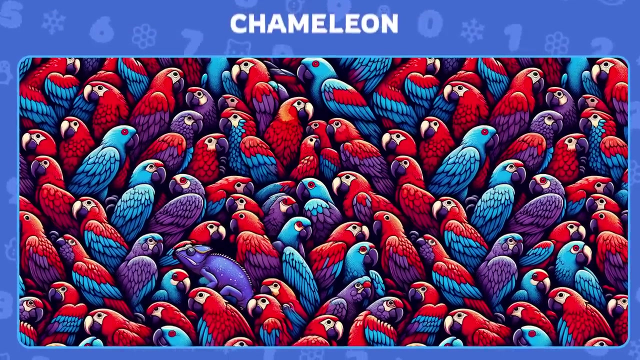 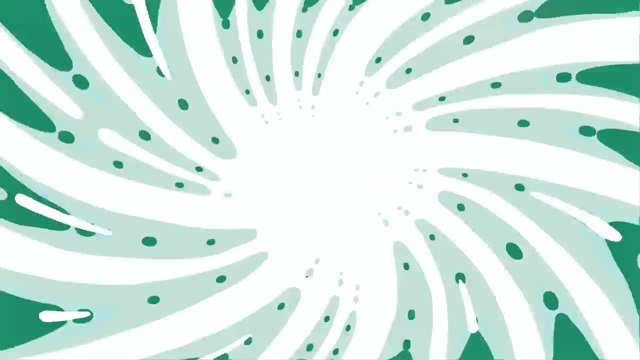 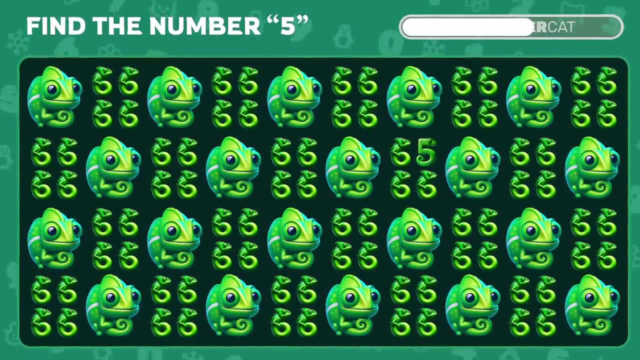 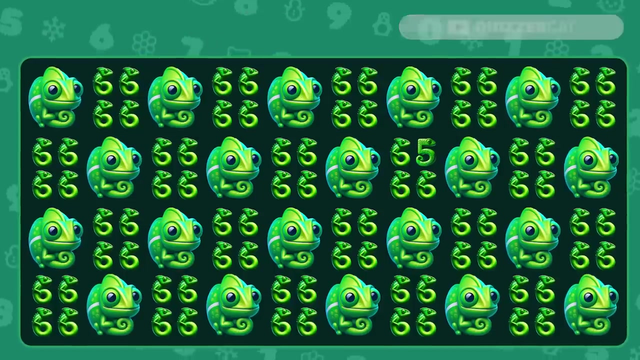 now the hardest levels. guess what's hidden among these lines? Yes, it's a parrot. look at all these colorful parrots. but there's another animal hiding, hiding. Can you find it? A chameleon is hiding among the parrots. Among these chameleons, try to find the number five. 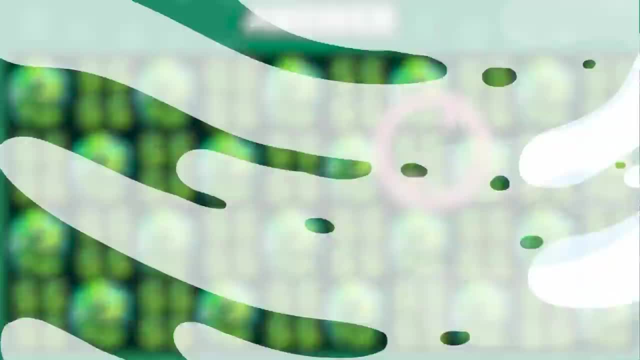 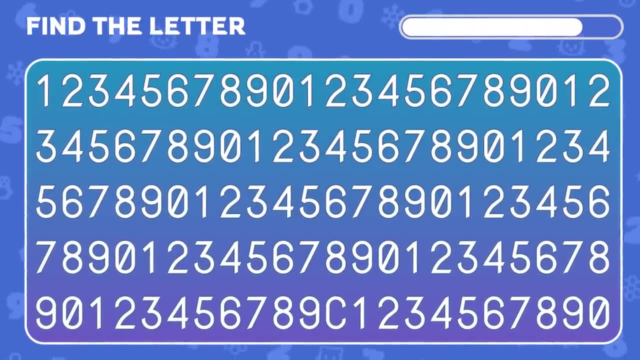 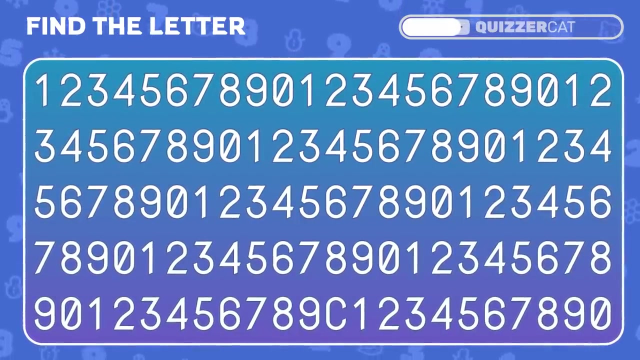 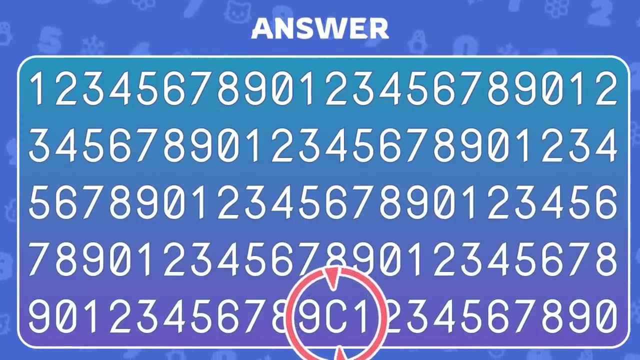 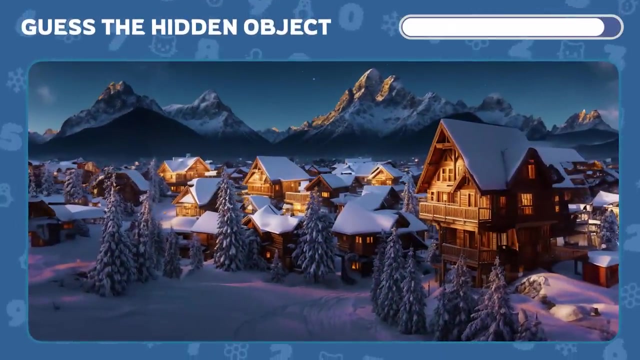 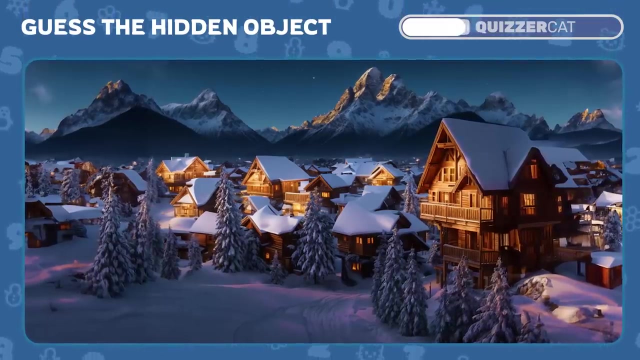 And there it is. Find the letter among lots of different numbers. Okay, A letter C is hidden among these numbers. Guess what's hidden in this optical illusion? It's the year 2024.. It's the year 2024.. It's the year 2024.. 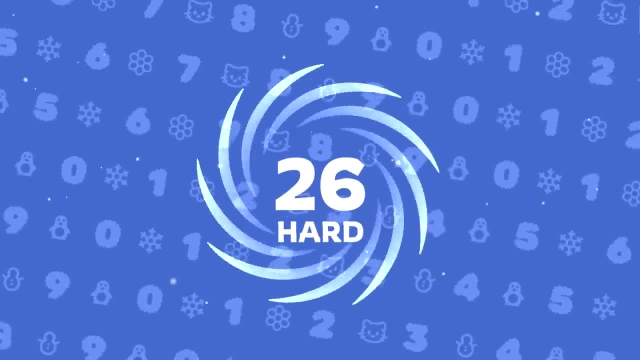 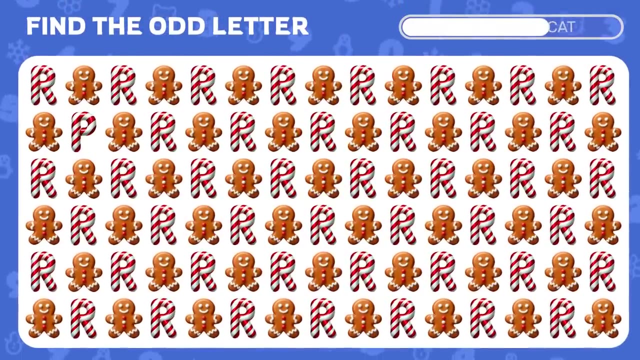 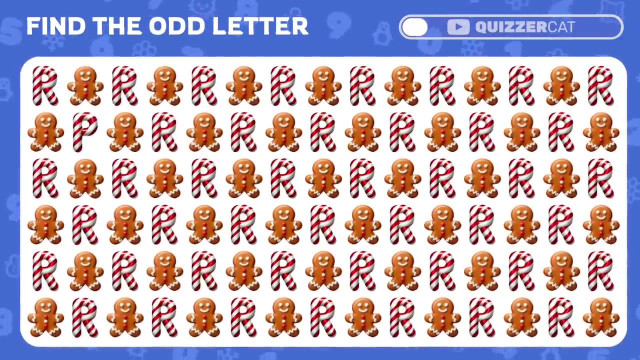 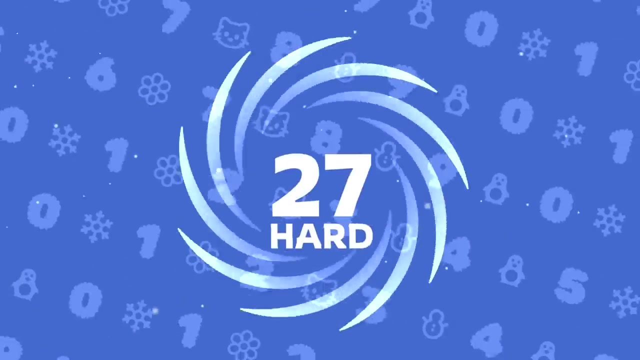 It's a lucky sixtieth. Find the different letter among these sweets. It's the letter P, located in the second row. A level for the sharpest minds. Find the emoji that doesn't repeat. I can't find it. See What's the rappers like to do. 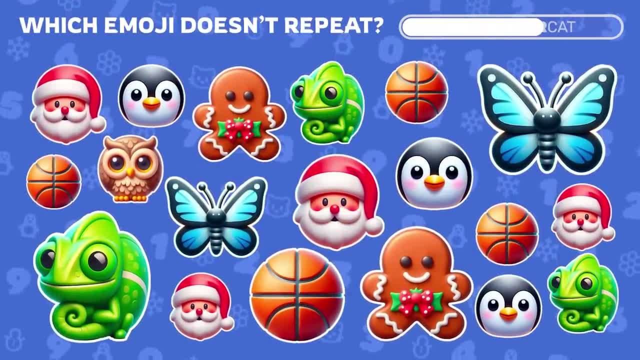 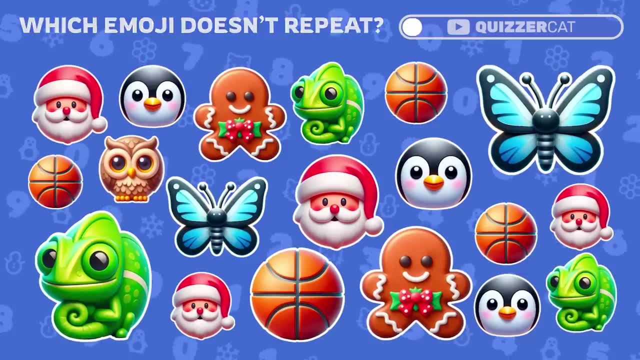 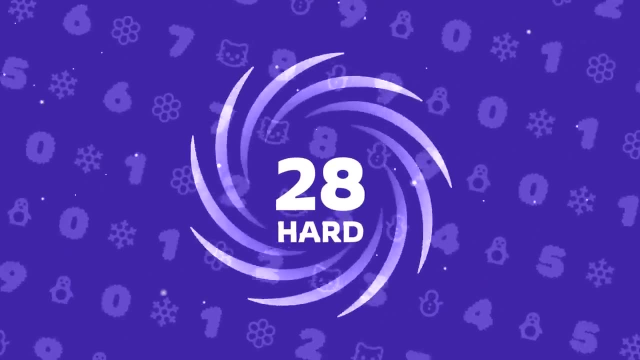 Can't find it, Let's find it again. Can't find it, Excuse me, Here we go. OK, there goes the second letter among these sweets. It's found, the letter P, located in the second row. The owl emoji appears only once. 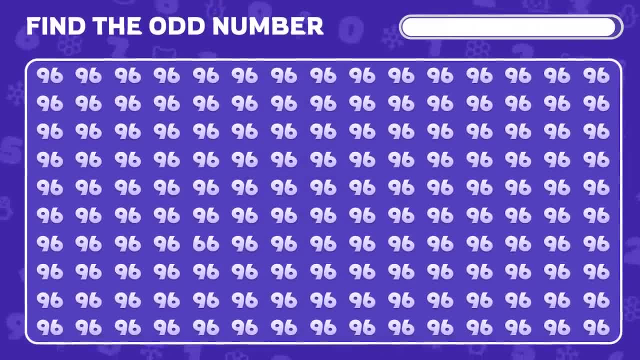 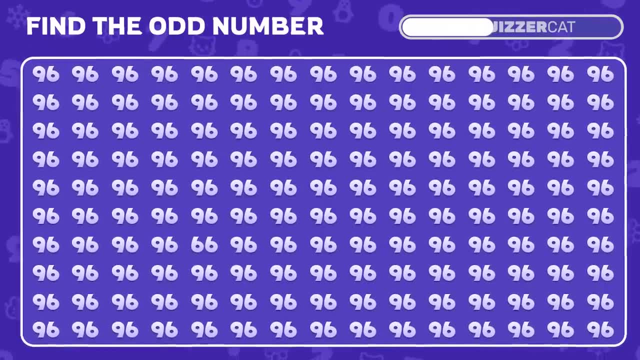 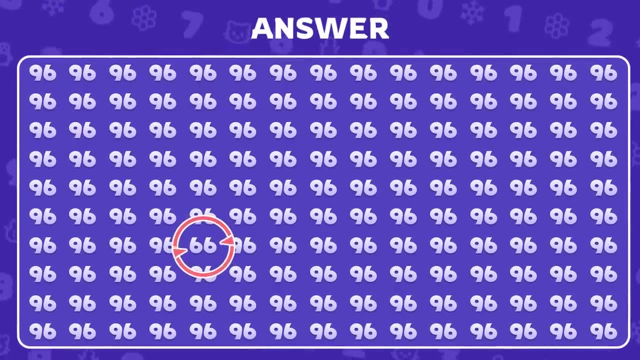 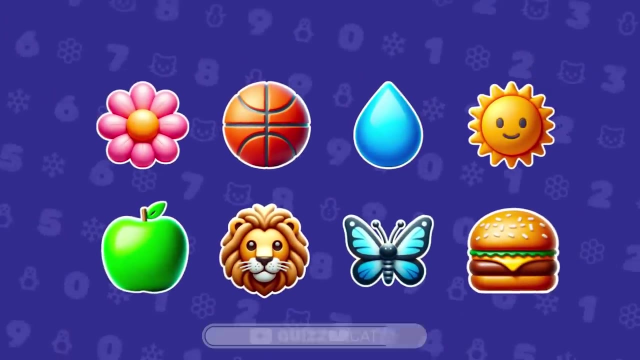 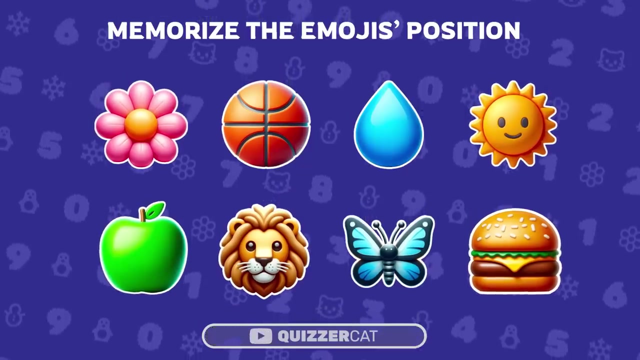 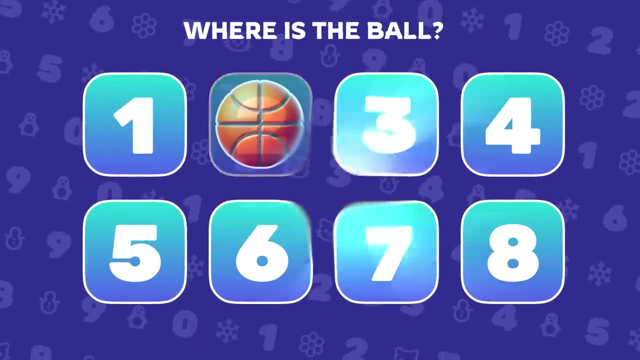 One of the most hardcore levels. Can you find the different number here? Wow, it's the number 66.. Memory test: Remember the positions of all eight emojis. Okay, Ready, Where's the ball? Yes, the ball is under number 2.. 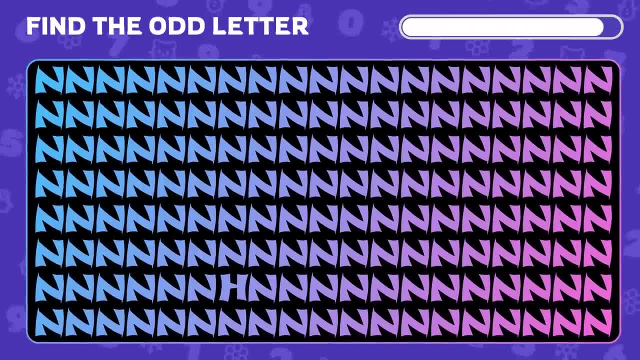 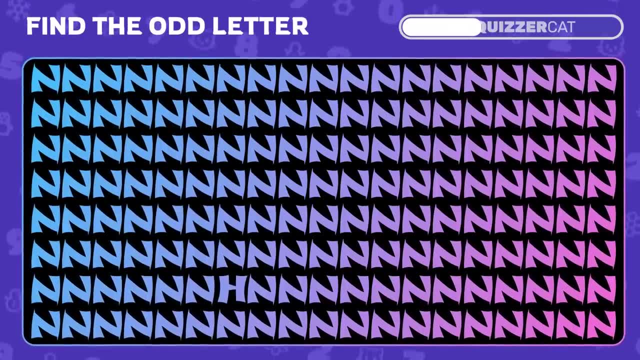 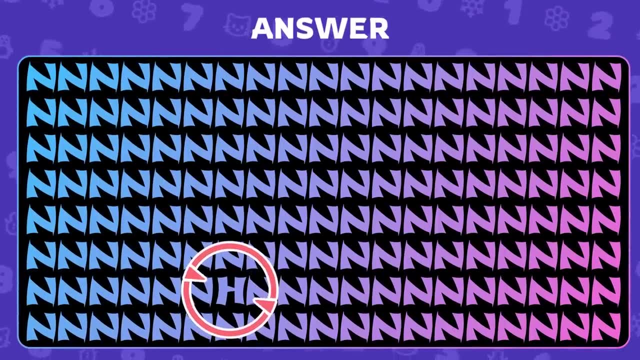 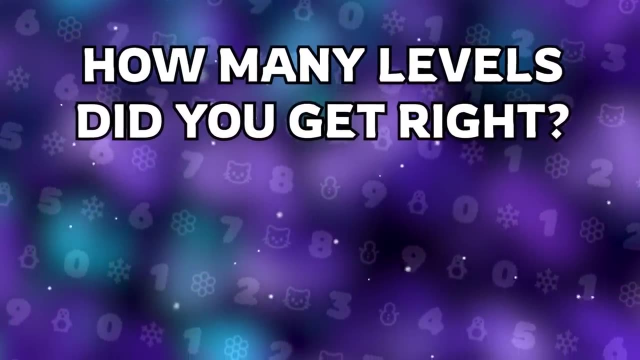 Finally find the different letter here. It's the letter H: Ready, Let's go. Great job, friends. Write in the comments how many levels did you get right, And don't forget to subscribe to see more exciting quizzes. Pick your next challenge. See you in the next video. 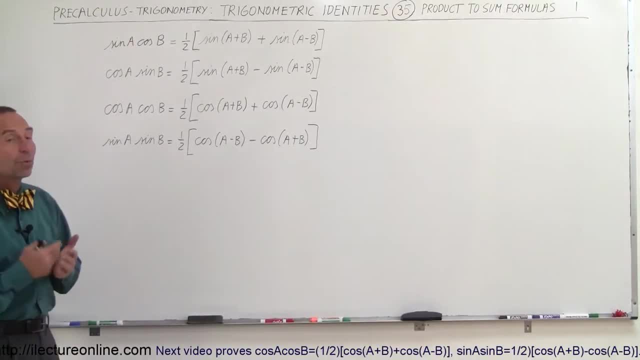 Welcome to Electoral Line, and now we're going to take a look at what we call the product. to sum formulas, Sometimes we end up with something where we have the sine of A times the cosine of B, or the cosine of A times the sine of B or the cosine.